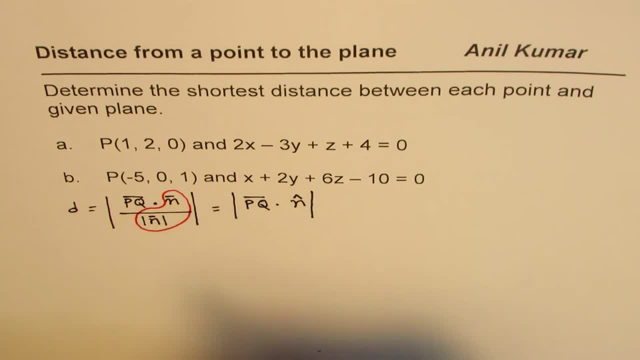 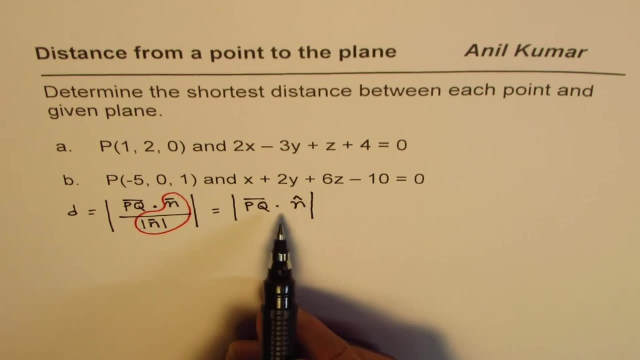 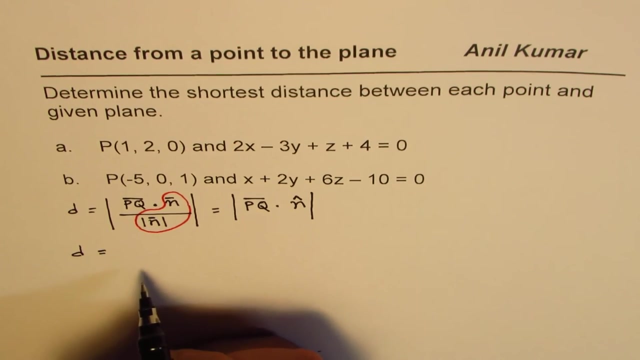 direction of the normal for the plane. Now, that is actually the definition, how you get the plane also, And we also have a formula which we will discuss in the next lecture. Thank you, This is a simple formula which many of the students will be using and that is much simpler. 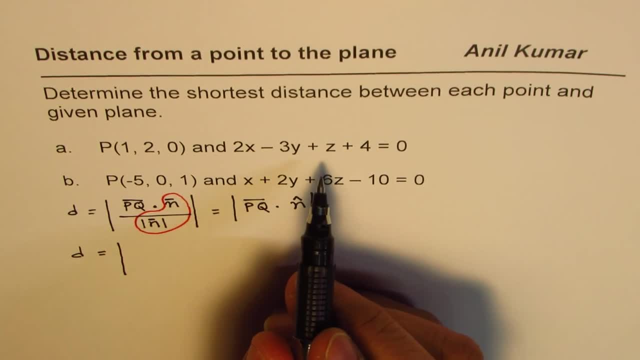 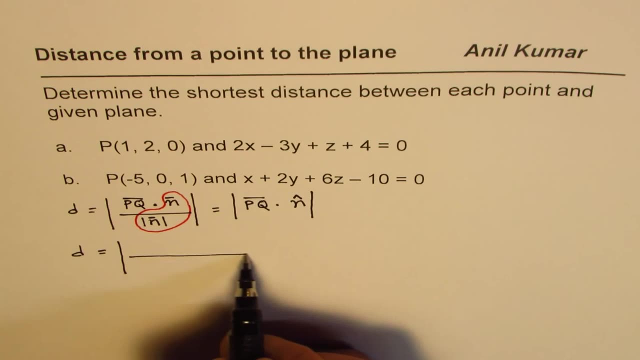 to use, especially when you are given an equation of the plane in this form right The Cartesian or the scalar form, And that is, you'll always find the unit vector kind of. I mean this as a denominator, which is a. let me write down the…. 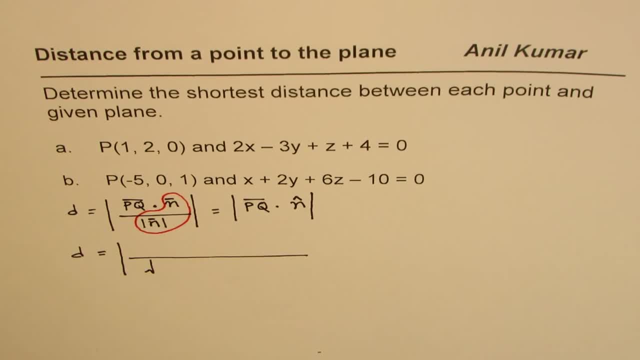 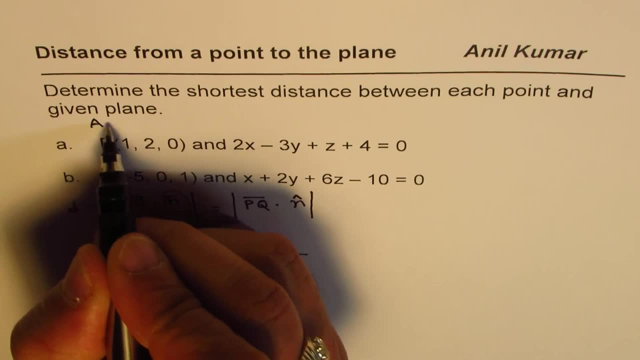 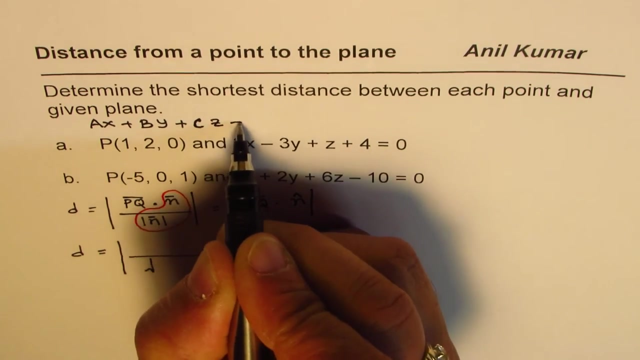 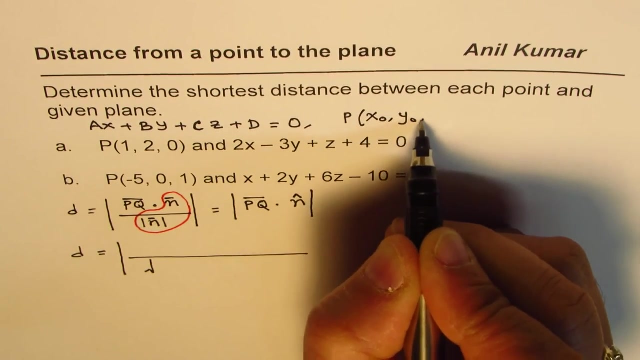 …. so so this formula, and let me write down general equation of the plane, which is: let's say ax plus by plus c, z plus t equals to zero. and let me write point p as x, 0, y, 0, z, 0, right. 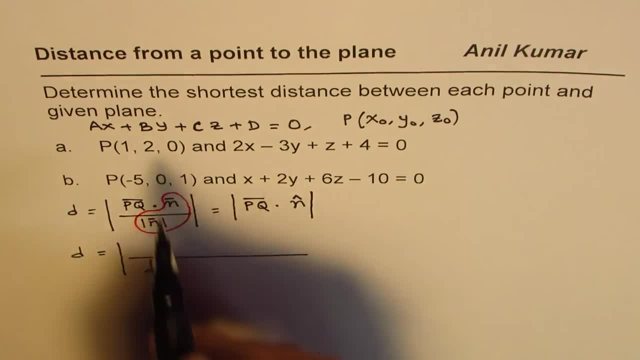 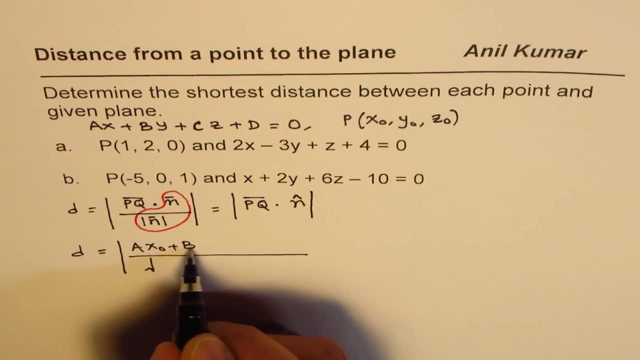 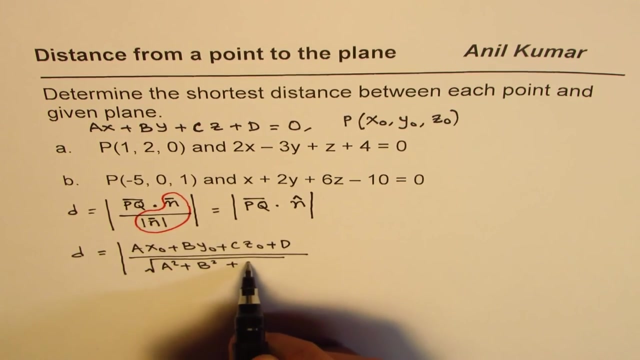 so our distance from this point to this plane could be written as substitute this value in the formula, which is ax 0 plus b, y 0 plus c, z 0 plus t right, and then divide by the normal, which is a square plus b square plus c square, the magnitude of normal right. so that's another. 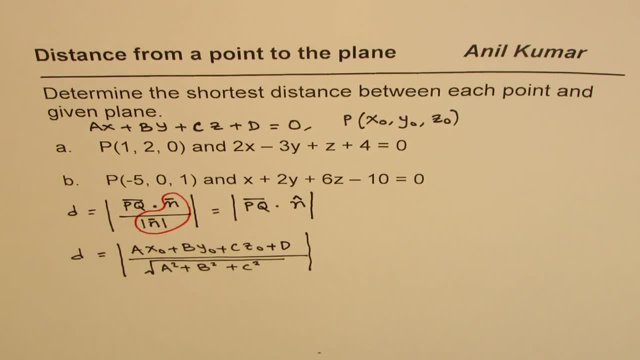 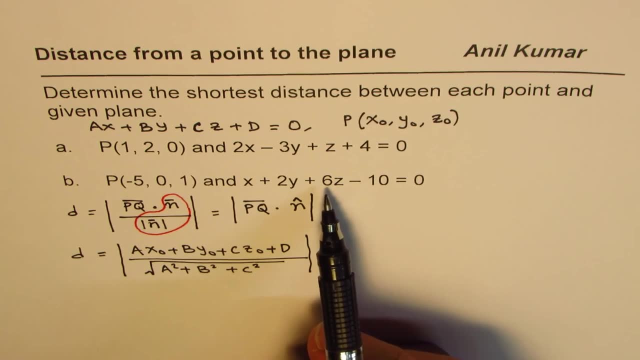 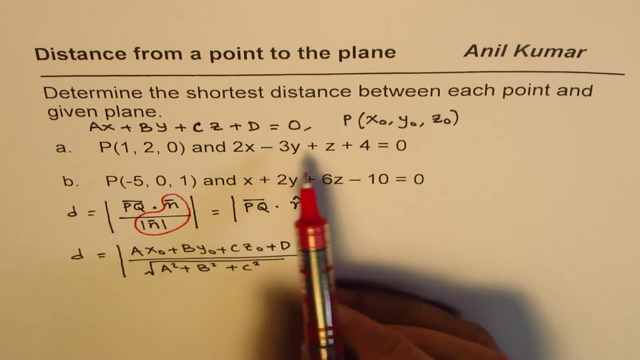 formula which can be applied to find distance. i'm sharing this with you because at different stages you may be asked this problem right, so that is how you should be doing it now. another important thing which i want to tell you here is that the first point here, may you know, the point may lie on the plane, and that's the. 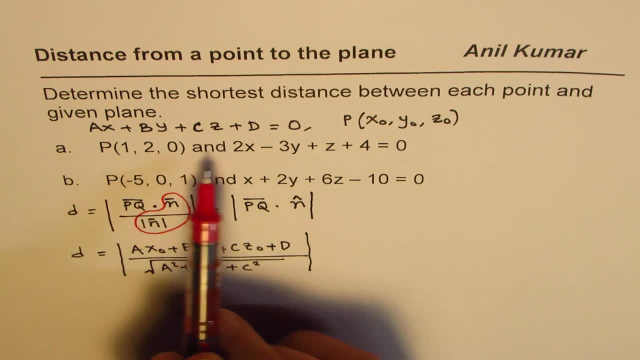 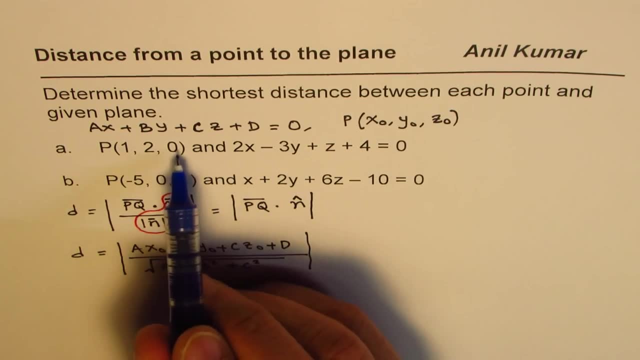 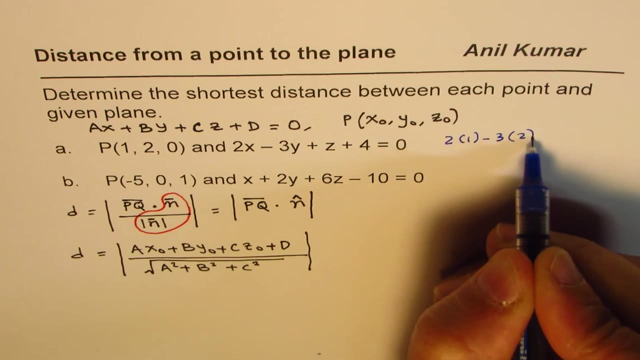 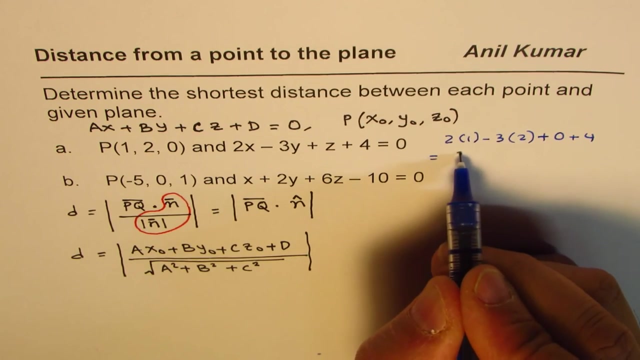 reason why i've given you this a see. if i substitute the point here, that is to say if i write: write x as one, y as two, zero as z, what do i get? i get two times one minus three, times two plus z, which is zero plus four, and that is equal to two minus six plus four. indeed, 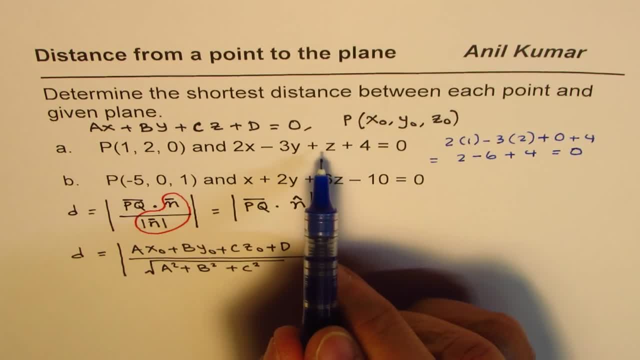 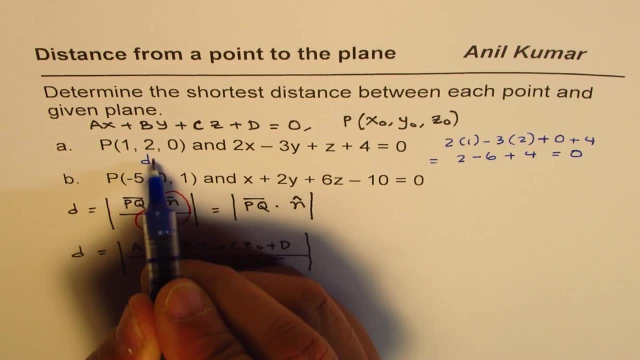 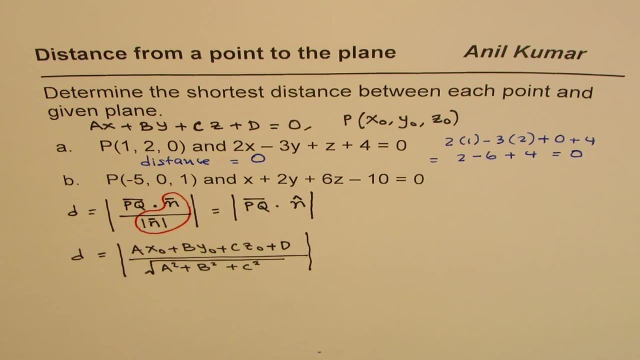 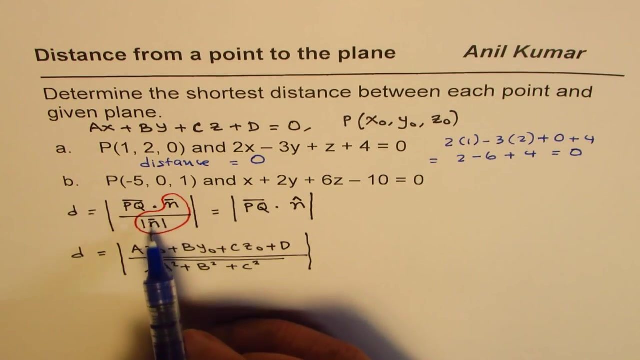 it is equals to zero. so this point satisfies the equation of the plane. that means the point is on the plane and therefore here, in this case, distance equals to zero, since the point is on the plane. so the idea of sharing all this with you is that, even before getting into all these calculations, 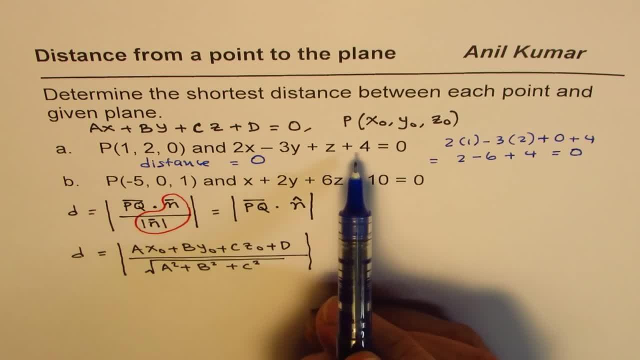 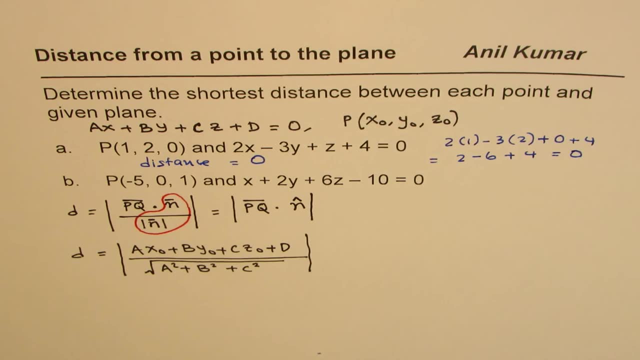 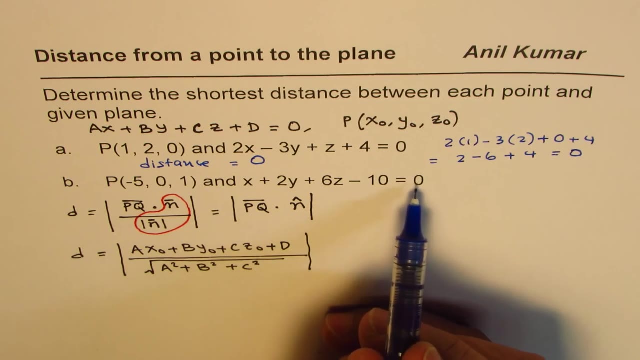 in the test, it's a good idea to check if the point is on the plane or not, right? that kind of helps us, since you have calculators and it's a very easy calculation, right? so so the next one here is: x plus 2y plus 6c minus 10 equals to zero. we can substitute this point. 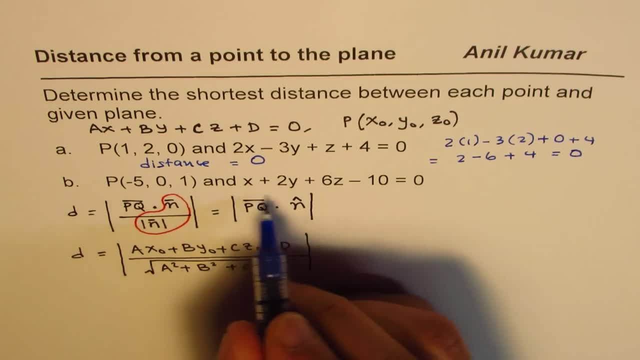 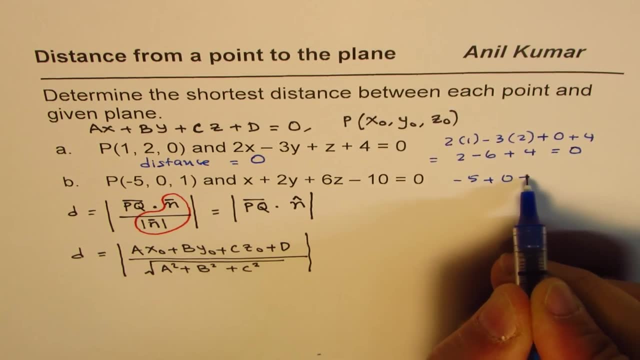 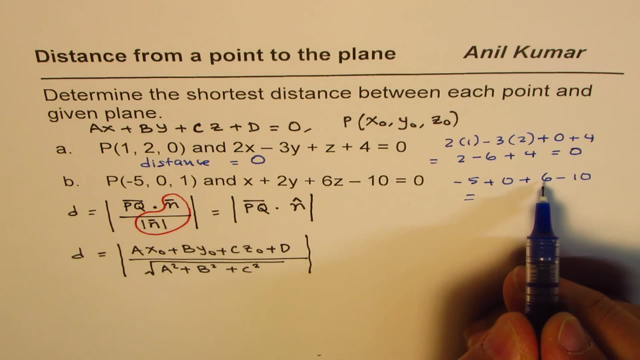 so we get: if I substitute this point, I get: x is minus 5. let me write: minus 5 plus 0, plus 6 minus 10, right, and then let's find what this is: minus 5 plus 6 is 1 and take away. 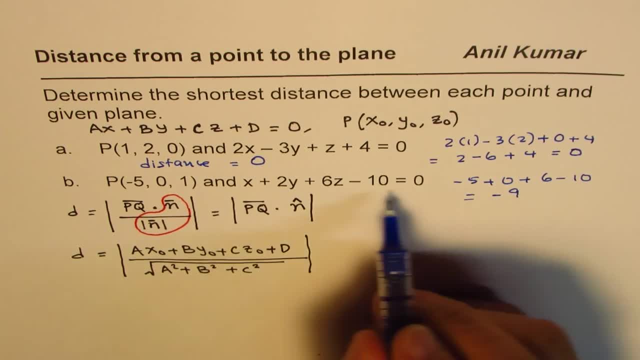 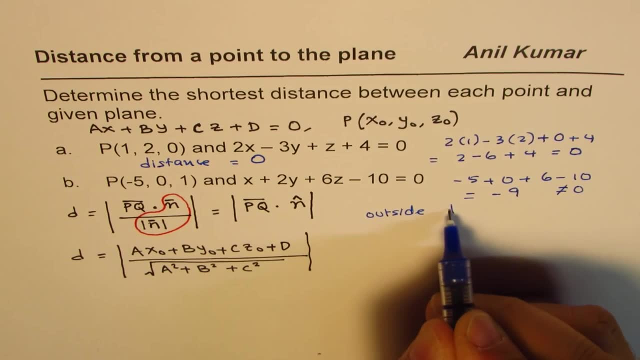 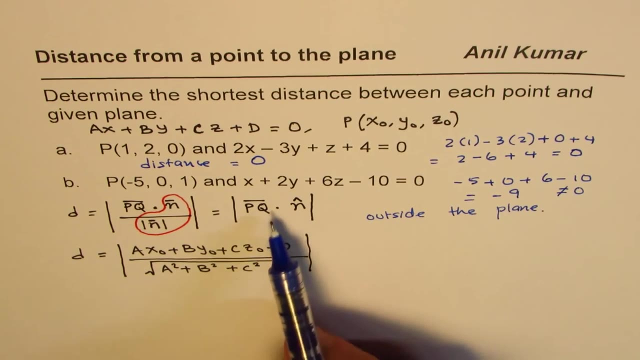 from 10 is minus 9.. Now this is not equal to 0, right? so this point is outside the plane, correct? so it will have some distance from the plane. so apply the formula whichever required and then get the answer. but the idea is always: 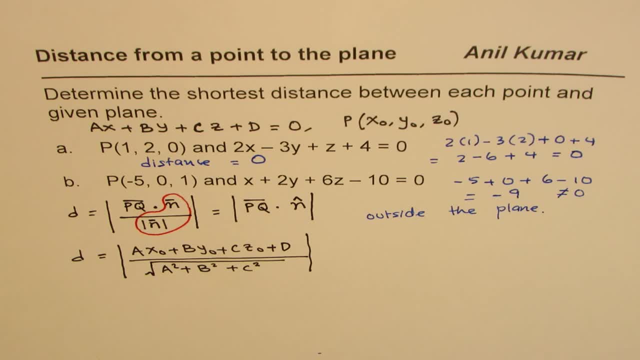 test if the point is on the plane or not. it really helps if you are doing some multiple choice questions correct now. this formula takes some time to solve, but this is a data based formula to apply, so we should apply this in most of the cases. right, so we are. 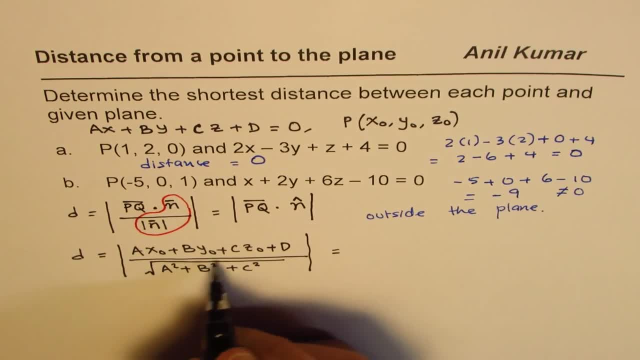 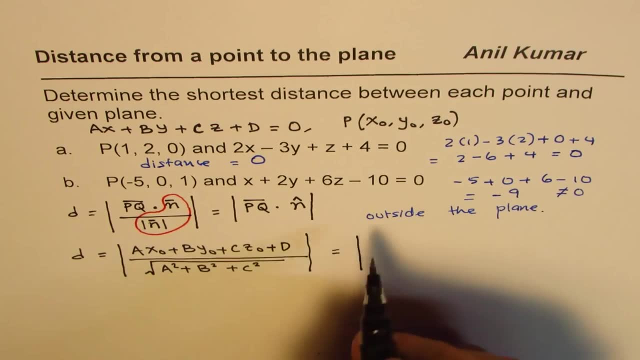 now find. we know the distance for a is 0 and let's find for b. so we already substitute this value. we got that, but anyway let's rewrite. so we'll write this as a is one for us, substituting the points to get minus 5 plus 2 times zero, minus 6 times 1 minus 10, so that we get the. 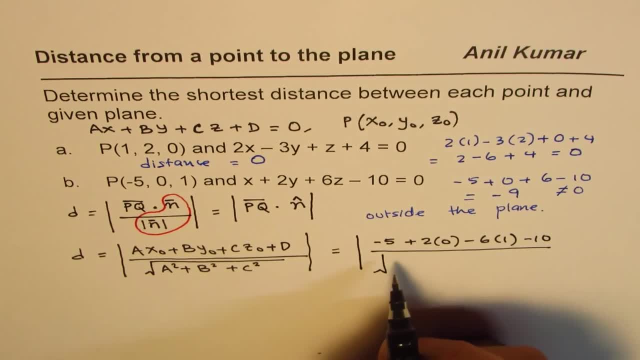 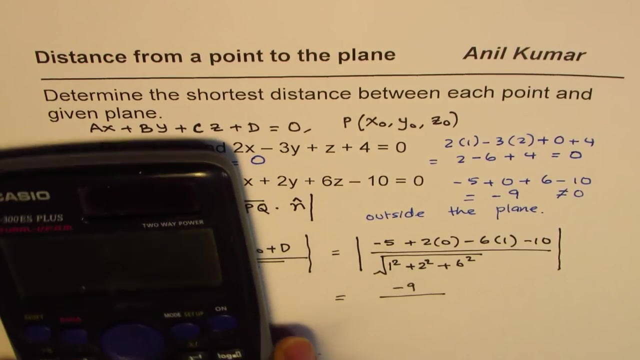 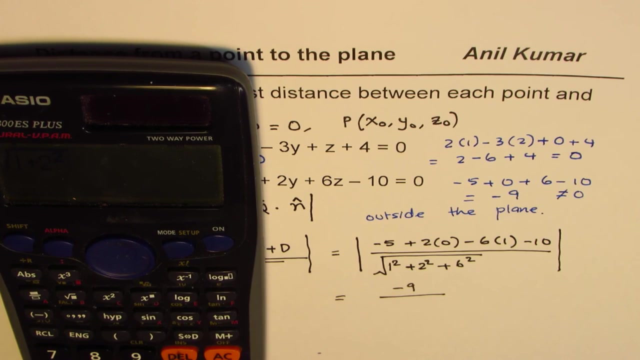 new part divided by square root of the normal vector, which is 1 square plus 2 square plus 6 square square root right. and that gives you, we calculated the numerator is minus 9 over. we can use the calculator to find the denominator which is square root of 1 plus 2 square plus 6 square equals 2, which is square. 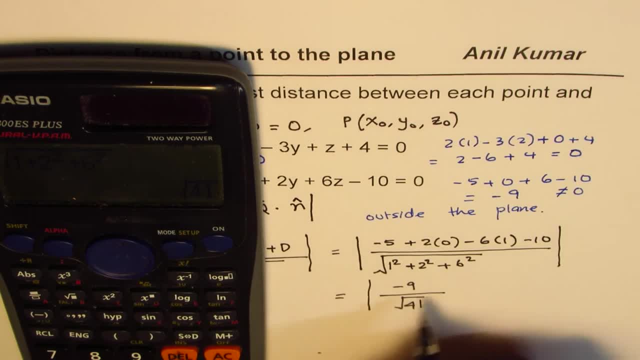 root of 41. right now, since always distances are positive, you have to do like this great absolute value, right? so that becomes your answer in decimals, if you really want to write will be 9 divided by square root, 41. you write in decimals. it could be equals to approximately 1 point 4, right? so you? 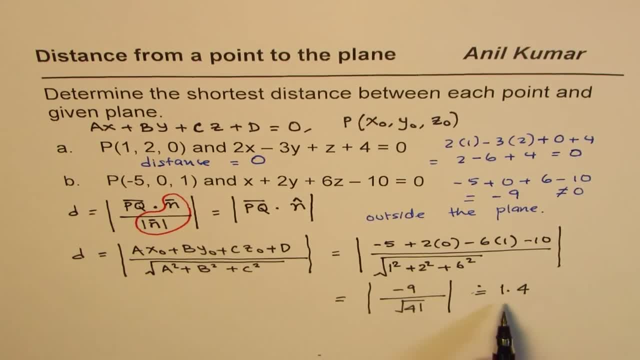 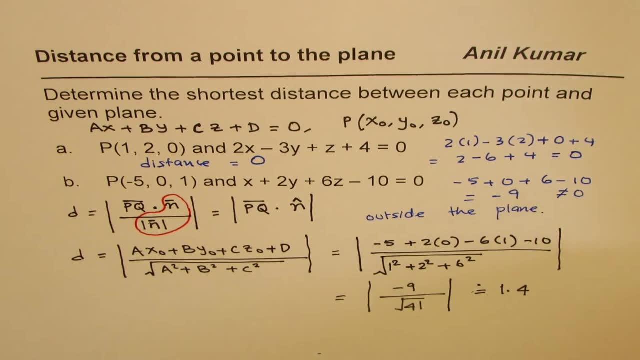 could answer like this also, right, so I'll see this, apply the formula and do it, and let me also give you the foundation for this formula. this formula really talks about a plane which is, let us say, kind of like this and let's say we have a point. 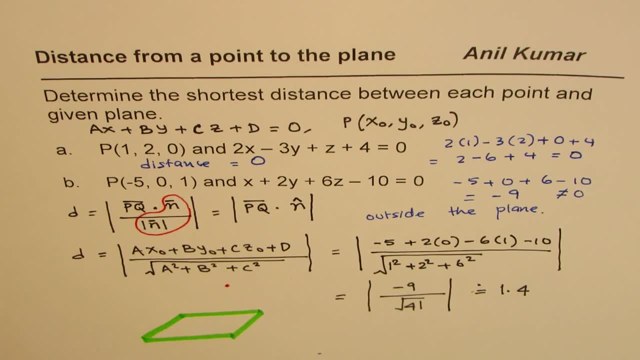 here. so distance is always the shortest distance which we are talking about will be normal, along the normal, to the plane, right? so that is the whole idea. so distance is along the normal. so this line, which is, which is perpendicular to the plane, will give you the distance d. 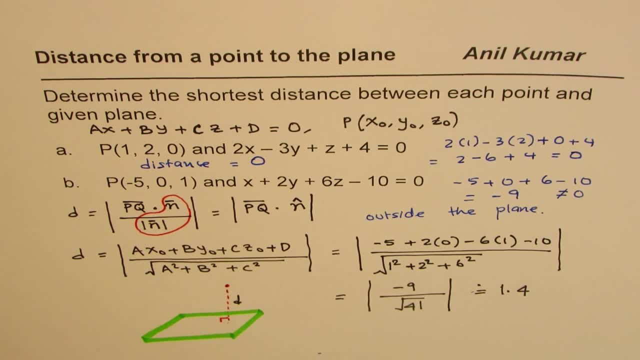 right. but it is very difficult to find the foot of this perpendicular. so what we do is we take up any other point and we call that point as q and this point is p given to us, right. so we just take convenient point p q on the plane and actually find pq, which is this pq dot product tells us. 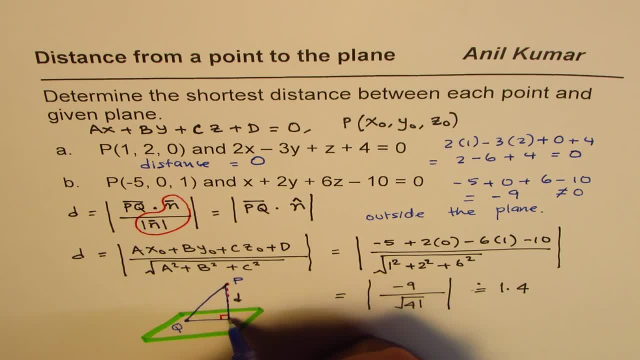 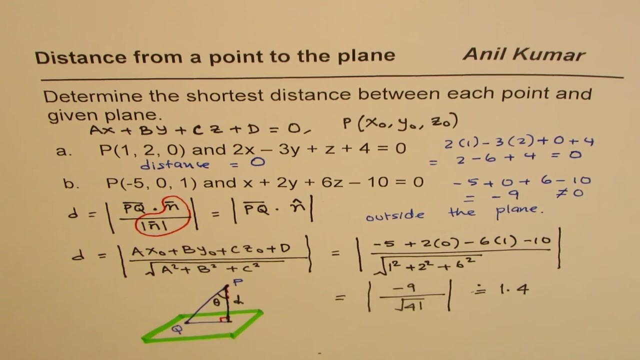 it's a component a along this direction. do you see that? so in this triangle, in this triangle, if that is the angle theta, then the dot component is the cosine, cos, theta, which is along this direction. right, that gives you the component of pq along this direction, gives you the distance, and that is. 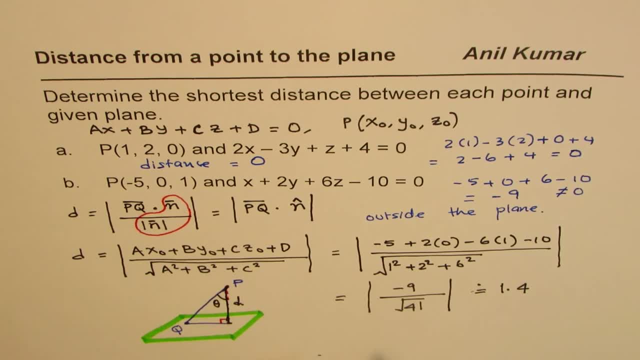 how it works, correct. so this is a good formula to apply and q should be selected as a convenient point, right? for example, in this particular case. let me redo this: in this particular case, q should be selected as you can say: y and z is 0. so what is x? x is 10, so we can say q is 10, 0, 0, right, so you? 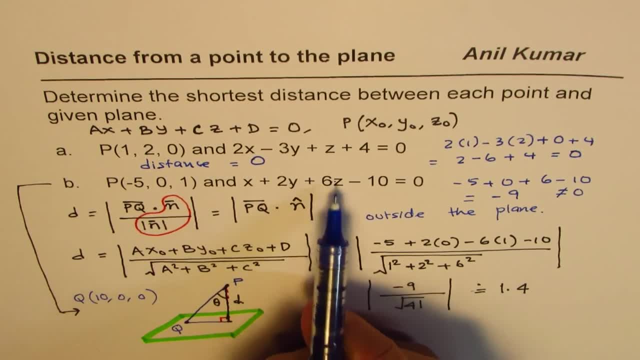 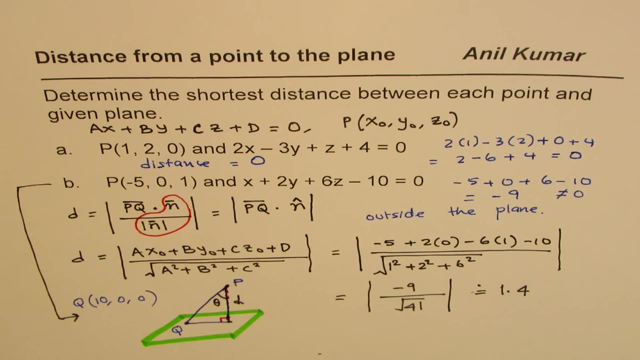 could select q as a very convenient point, placing zeros for y and z. x is 10.. once you know that, then you're gonna apply this formula and check the distance right, all right. So I think it helps to understand when to apply which formula, and even before applying. 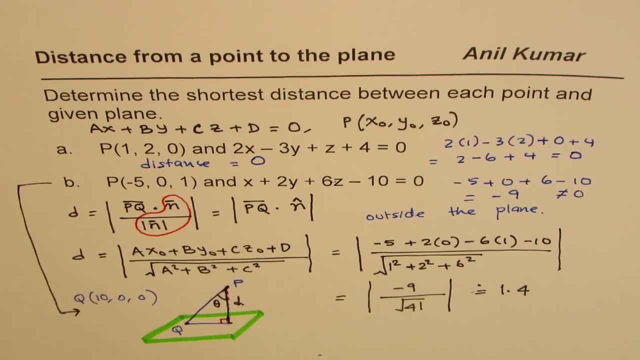 a formula, we should actually check whether the point is on the plane or not. Now, if you are using this formula, then check is not required because you will get zero in the numerator and you will know that the point is on the plane. but in case you are, 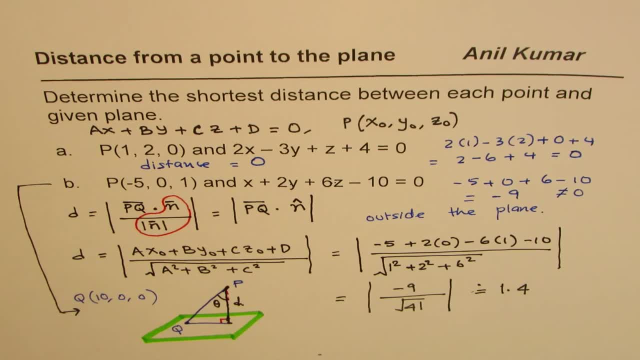 applying that formula. it helps. So it's a word of caution. I'm Anil Kumar and I hope that helps. Thank you and all the best.